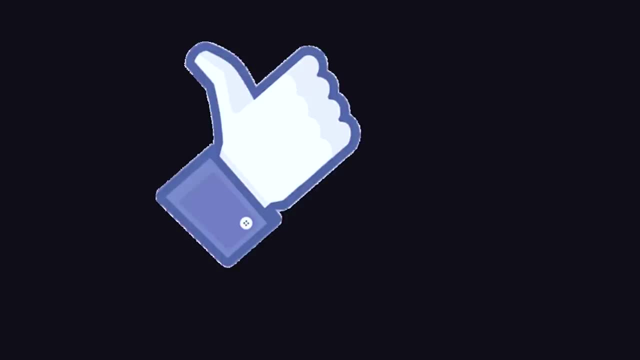 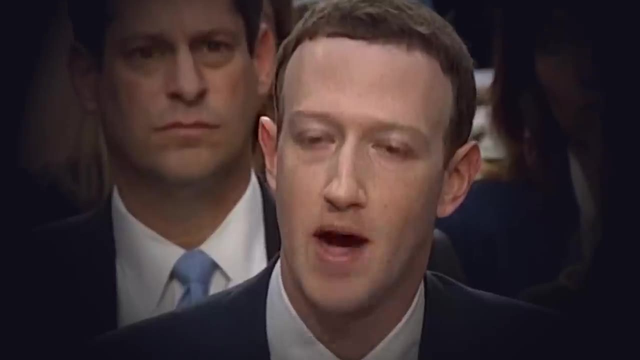 Reactjs, A half-baked functional UI library created at Facebook that's used by millions of developers because it has a cool name and logo. It was invented by Mark Zuckerberg in 2013.. And that was a big mistake And it was my mistake And I'm sorry. 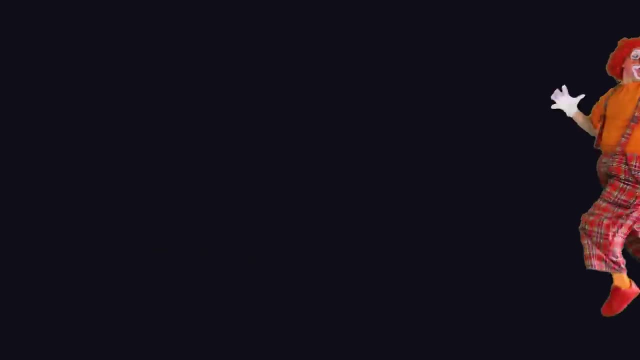 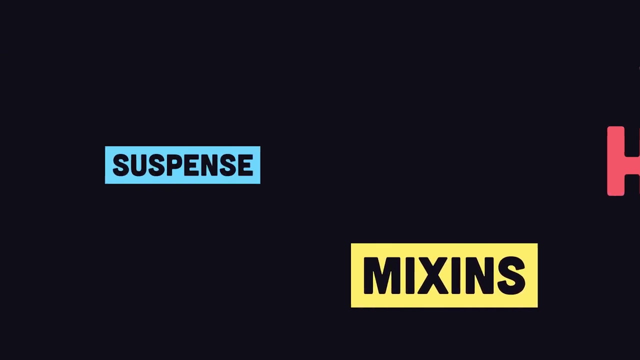 React is simple. It's just JavaScript, bro, And that's why it gives you dozens of weird ways to solve the same problems, like functional and class-based components, hooks, forward, ref, higher order components, mixins, render props, suspense, and so on. It's credited as the first. 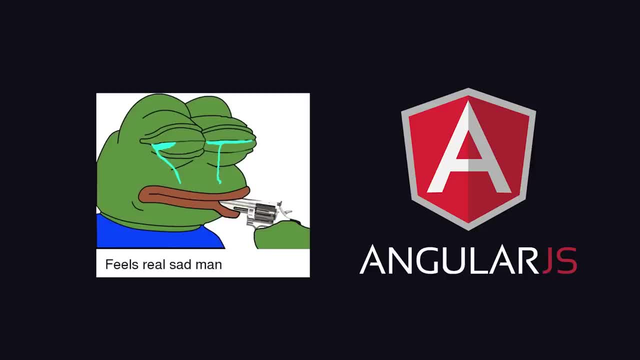 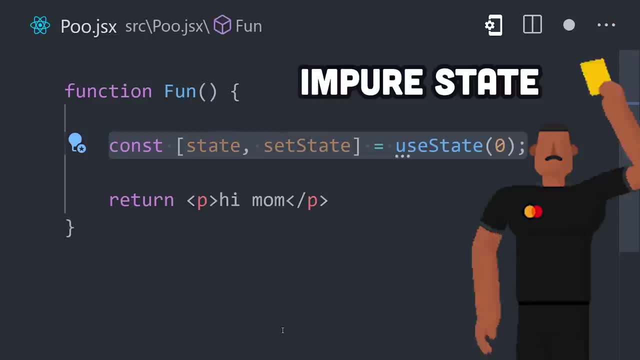 declarative UI library, even though it took most of those ideas from AngularJS. Its killer feature, though, is the fact that you can write pure functional code, That is, until you want to do anything useful, in which case you'll need to write impure functions with state and effects. 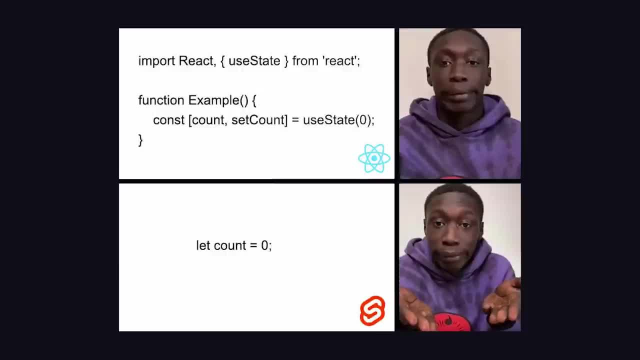 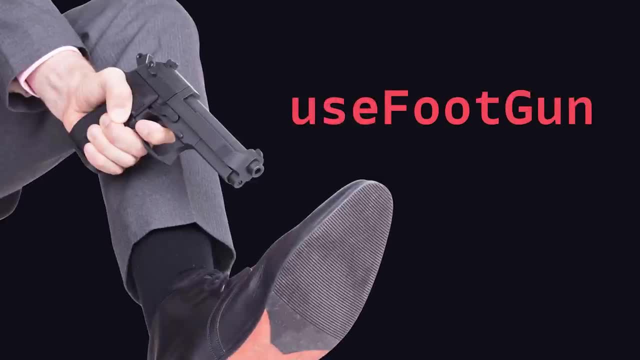 The beauty of this approach is that it makes simple things like reactive state much more complicated than they need to be, And that's what makes us feel like real developers. UseEffect is especially fun and was originally going to be called UseFootGun, because it's a great way to 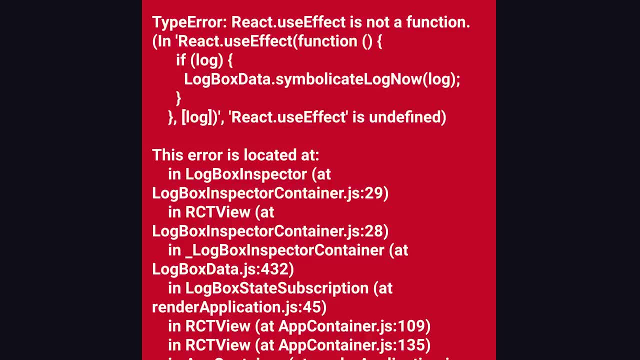 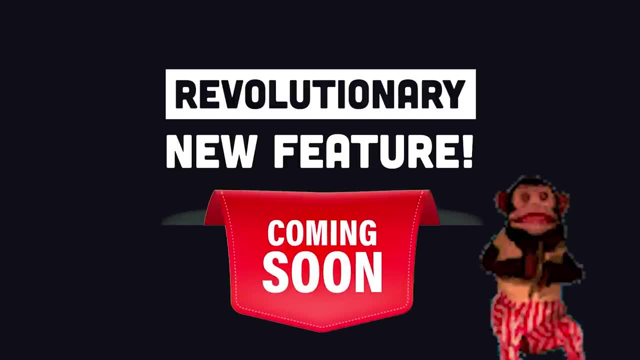 introduce infinite loops, performance issues and bugs that you'll never be able to figure out. Not to worry, though: React is always evolving with revolutionary new features to monkey patch all the weirdness nobody saw coming on the previous release. Now, even though it has an extremely high learning curve, React is a library. 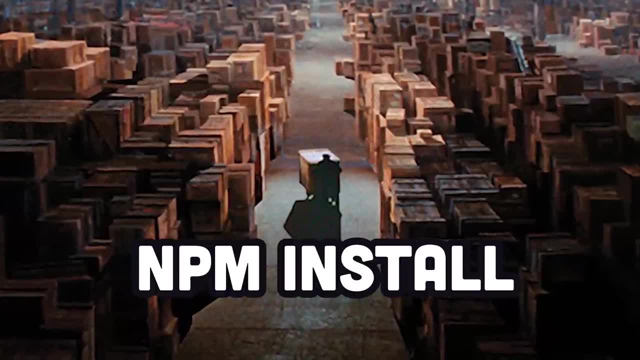 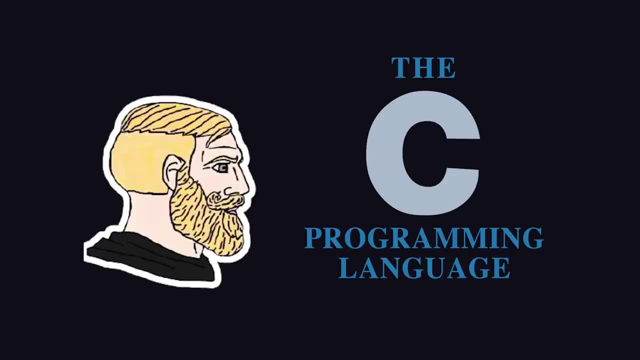 and not a framework, And that means to build something cool. you'll need to find and install hundreds of different packages, most of which were built by teenagers who stopped maintaining them years ago when they went off to college to learn a real language like C, To get started. 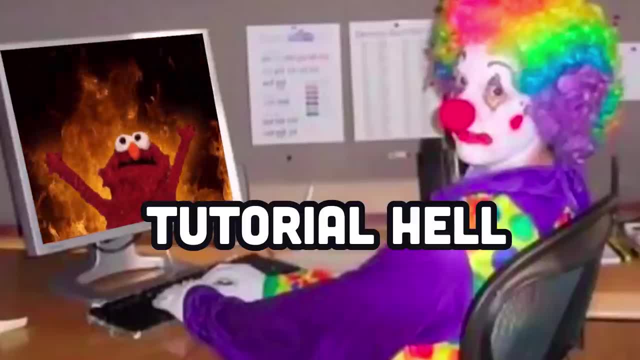 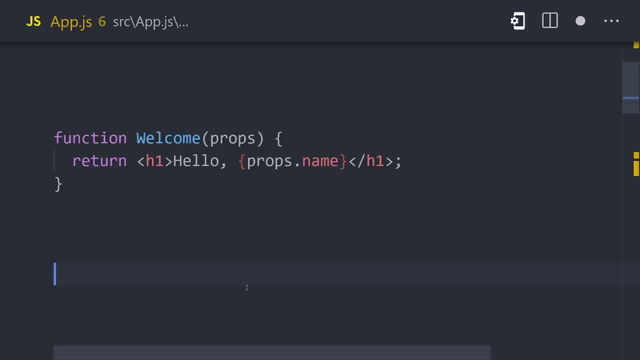 create a new React app, then open up Google to enter the gates of tutorial hell. Notice how we start in strict mode. That's used to hide baggage from previous versions of the framework. I mean library. Now in the code we pretend we're doing, 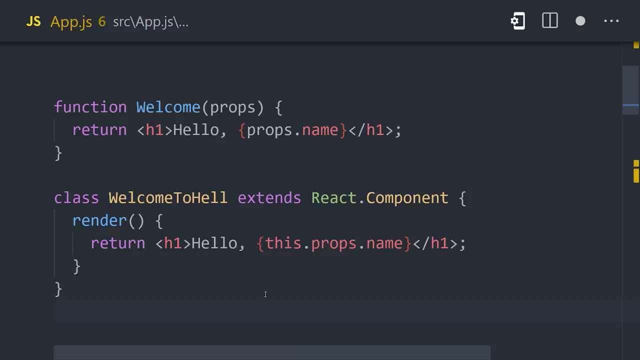 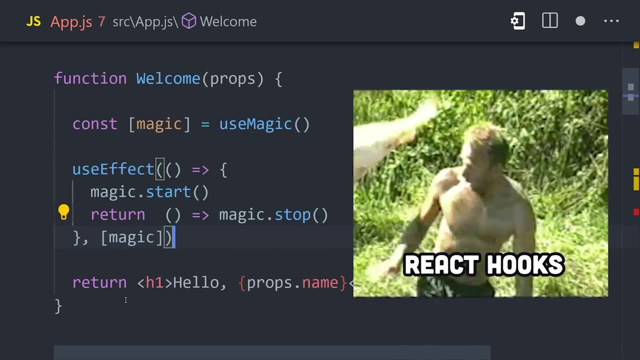 functional programming by writing our components as functions. Classes are also possible, but they are literally the devil. Instead, we use these hooks everywhere that do the same shit classes do in a more magical, hipstery way. Templating is handled in JSX. It's a non-standard way to write. 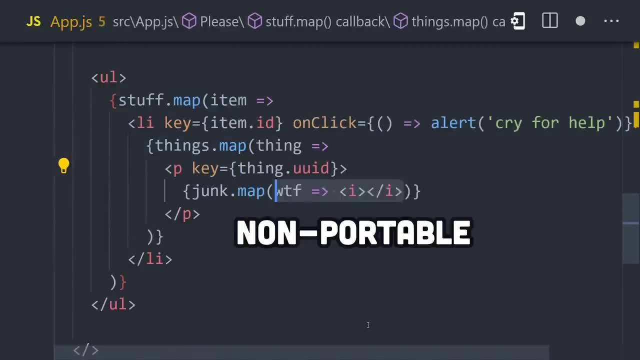 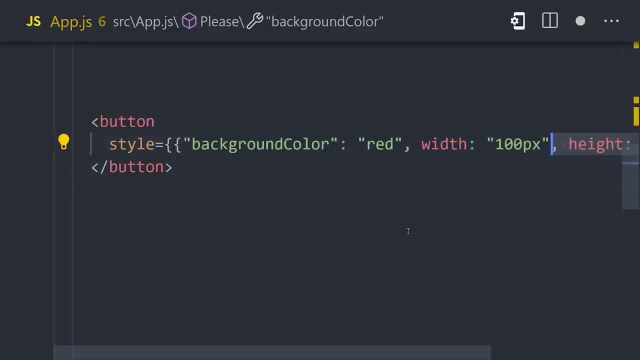 HTML which allows you to represent the UI entirely in non-portable callback. hell Now, we can all agree to hate CSS, but React will make you hate it even more when you try to style something on your own. Luckily, there are hundreds of CSS and JS libraries working on this problem.